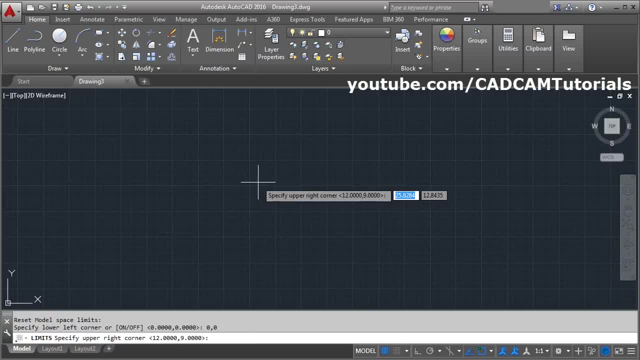 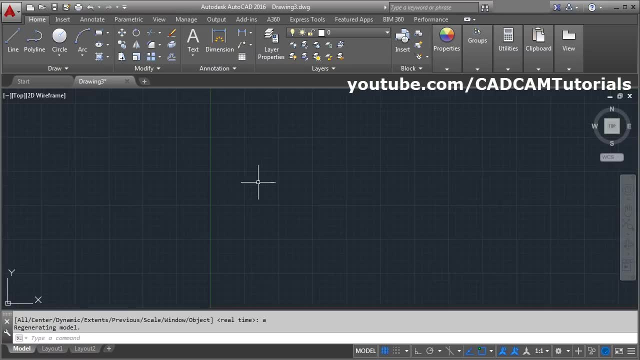 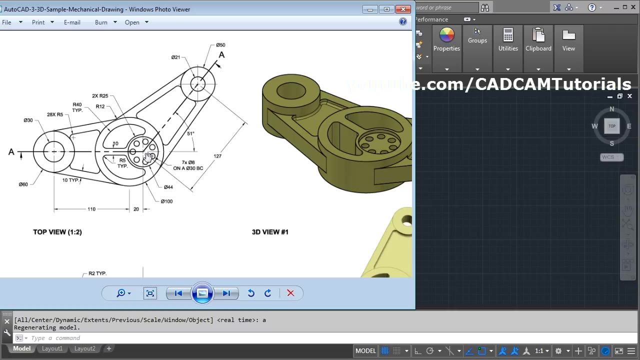 Lower left corner: 0 comma 0. enter. Upper right corner: 400 comma- 400. enter. Then give zoom all. Enter Z. enter A. enter At first. we will create this line of 110 and 20 and this 127 length in 51 degree. Take the line command, Give the first point, Make ortho on, Give the length of 110.. Enter, Then give length of 20.. Enter, Then make ortho off, Then give the length of 120.. Length of 127.. 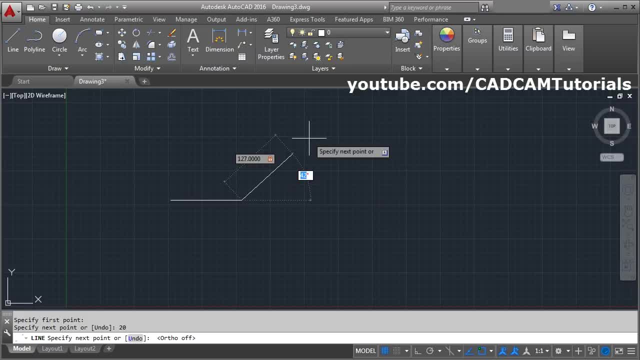 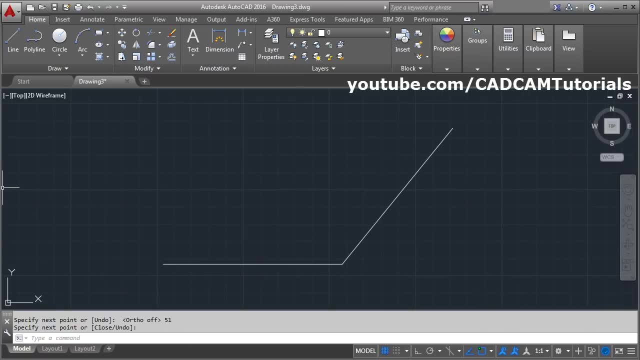 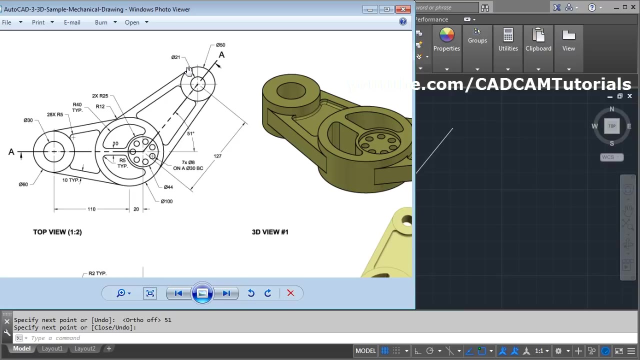 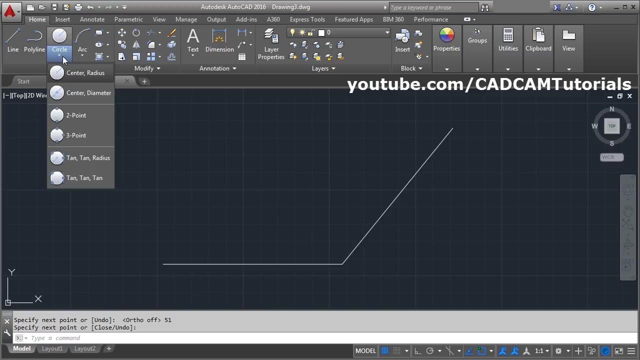 Then press tab for angle and give the angle of 51 degree. Enter, Enter, Zoom it. Here is two circles of 60 and 30 diameters and here are two circles of 21 and 50 diameter. Click on the arrow below the circle. 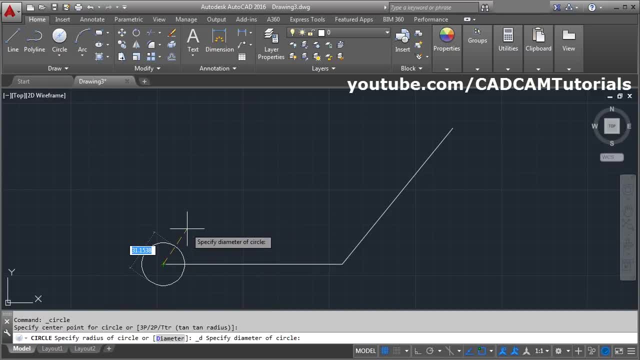 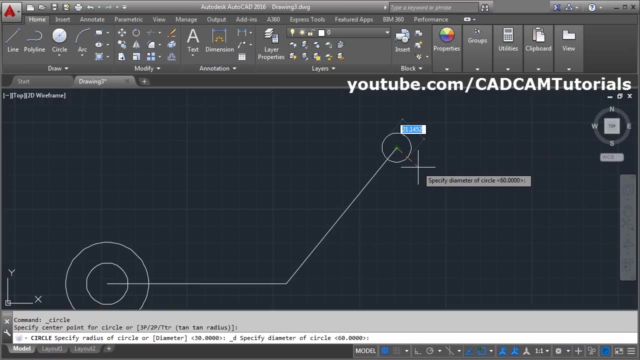 Take the center diameter. Give the center point, Give the diameter of 30.. Enter Again: click here. Give the center point, Give the diameter of 60.. Enter: Give the center point, Give the diameter of 21 and 50.. 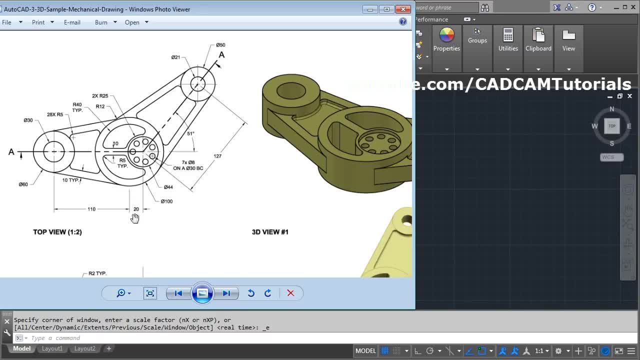 Then next is this circle of 100 diameter: Enter. Give the diameter of 120. Enter. Then click on the center point. Give the center point. Enter, Enter, Enter, Enter, Enter. Click on the center point. Give the center point. 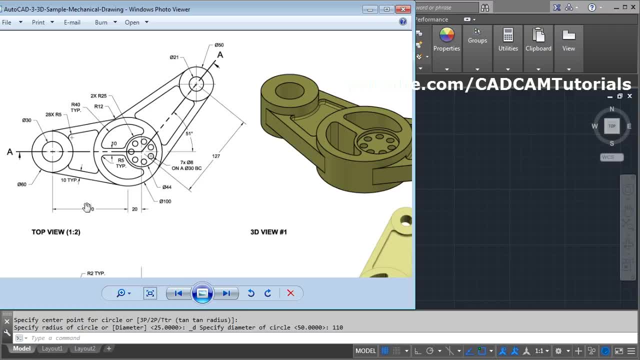 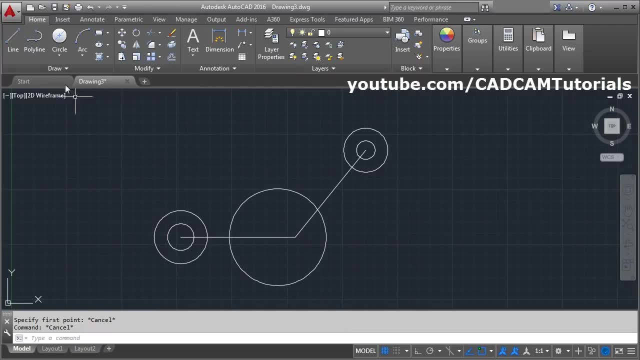 At this point give the diameter of 110.. Enter. Then there are these tangent lines. are there to this big circle from the smaller circles To create the tangent lines, take the line command. Now here it is showing the quadrant and center object snap. 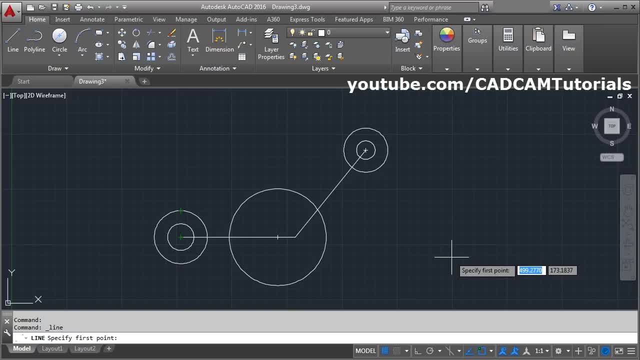 we want to give the tangent object snap. to activate the tangent object snap, click here, select tangent. now, here, actually it is showing the quadrant and not the tangent. in order to show the tangent we will have to make this quadrant and this center off. now take your cursor here, give the tangent point, give the other tangent point here, enter again enter. 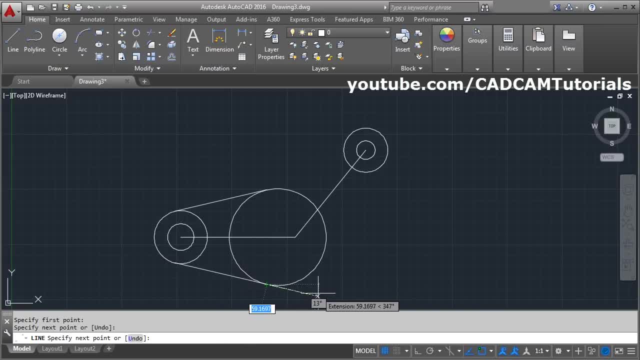 from here to here: enter, enter, click here and here enter, enter from here to here. enter, then here- actually there is a radius of 12- take the fillet command, click on fillet, then click on radius, give the radius of 12, enter, then select this line and select this line. now here is the radius of 12.. 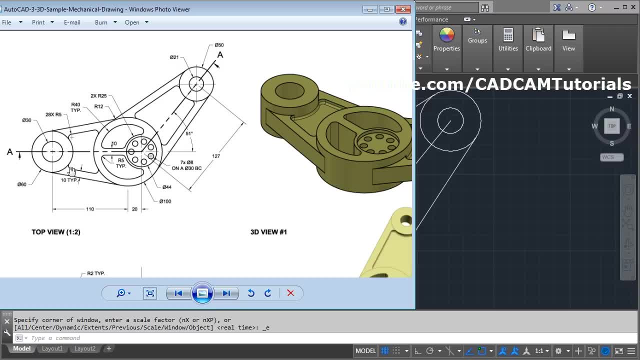 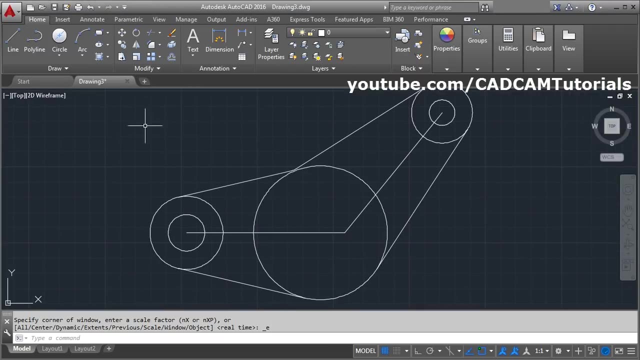 now. then next will be this portion: here is the gap of 10, same way here also the gap of 10, and same way on this sides also. we will offset it by distance of 10. offset, give the gap of 10. enter, select this line, go inside and click there. same way for all the other lines. take the line, go inside. 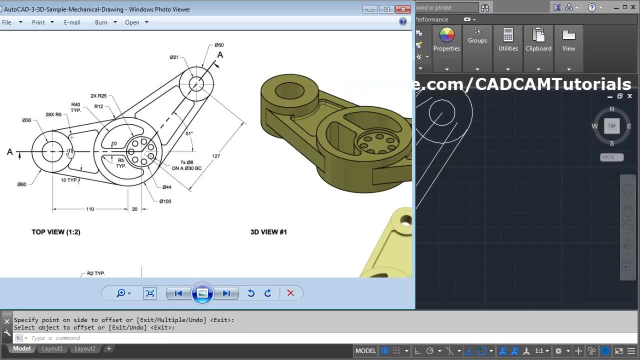 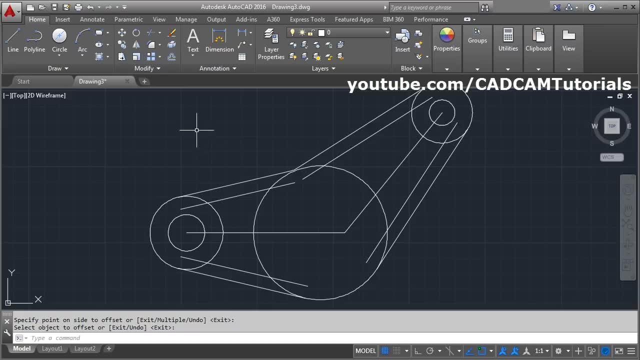 and click there, press enter. then at the corners there are the fillets of radius for you. again, take the fillet command, click on radius, give the radius of 5, enter and select this circle and select this line again enter. click on this multiple so that we can use this fillet command multiple times. select this line, circle, circle line. 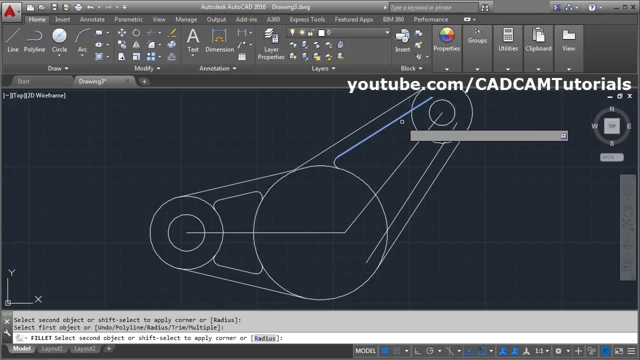 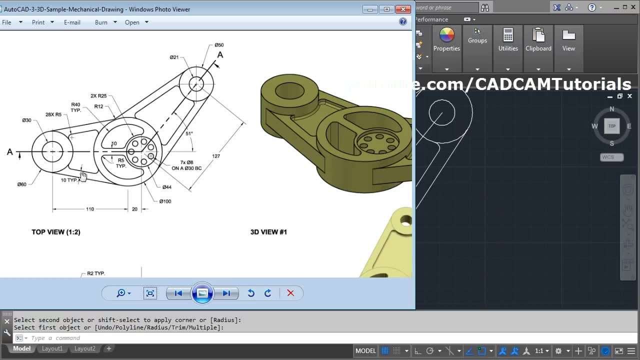 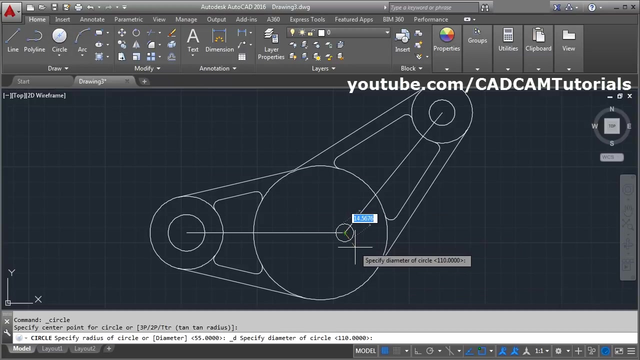 fill it all. the corners, intersect point. it will give the back portion and subtitle: now this portion is ready. then next is this inner portion. now here, this circle is of dia 44. create that circle center diameter. give the center point here and give the diameter of 44. enter. 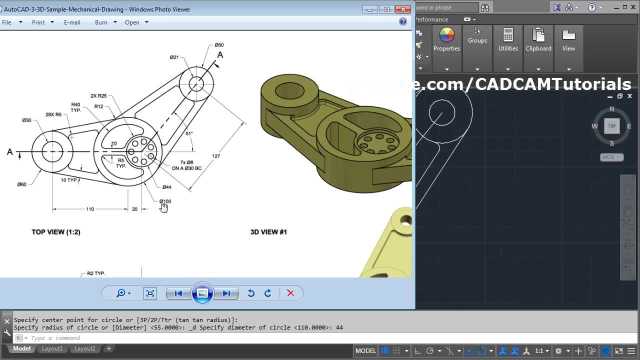 outside circle diameter is 100, that is radius is 50, this circle radius is 40. that means this gap will become 10. that means we will have to offset it by 10. inside, then here it is 44, that is radius is 22 and this radius is 25. that is, this gap will be 3 and here again the gap is 10. 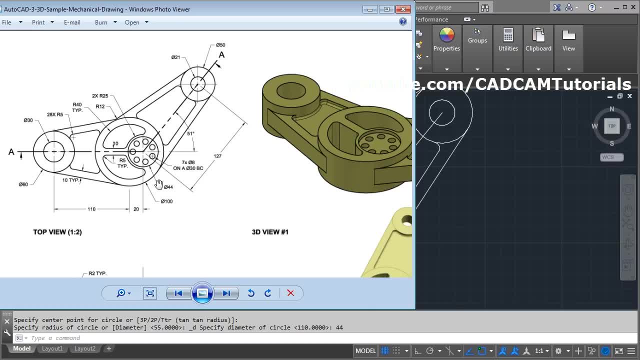 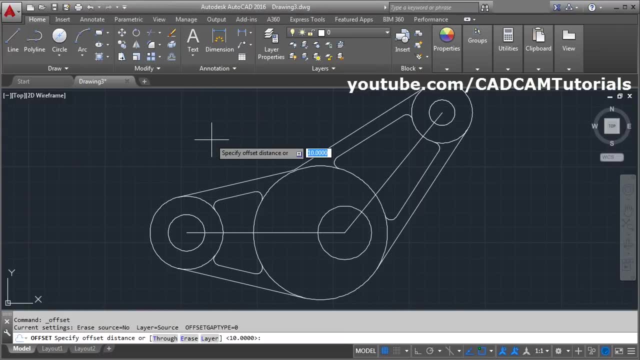 that is, 5 on either side. let's create this portion. select the offset, give the distance of 10. 10 is already there. press enter. select this circle. click inside. then again select this circle. give the gap of 3, enter. then select this line. take a bow and give the gap of 5. then this corner radius are: 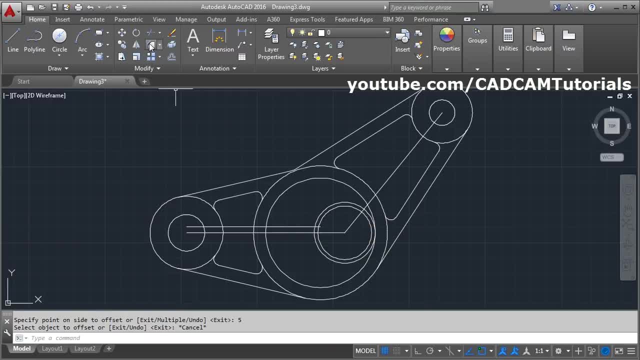 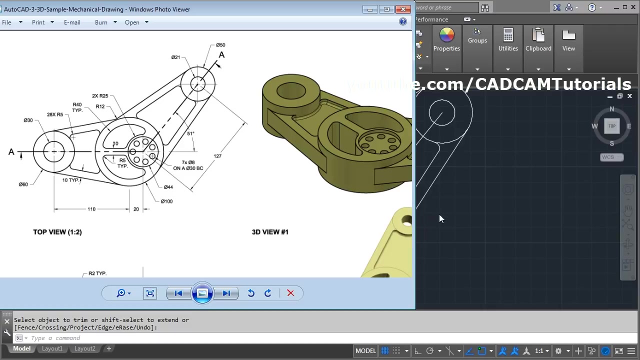 for you escape. then again, click on fillet. radius 5 is already there. click on the multiple and select this line, this arc, and complete all the fillets. enter, then trim the unwanted portion. give the trim command, press enter and remove the unwanted portion. enter: this shape is ready. then same shape is on the opposite side. we can mirror it. 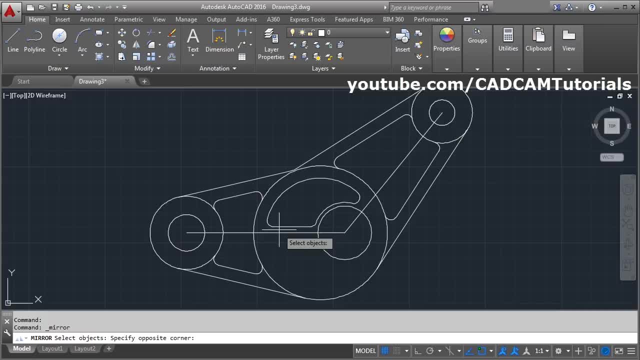 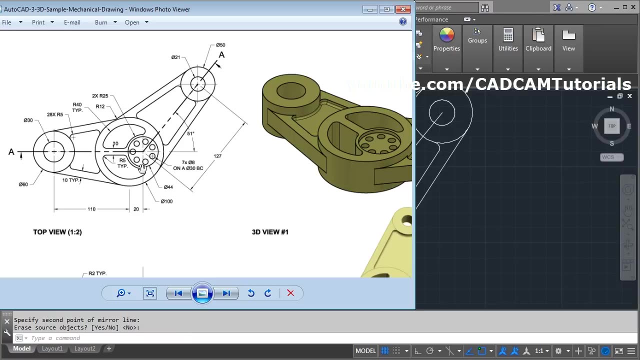 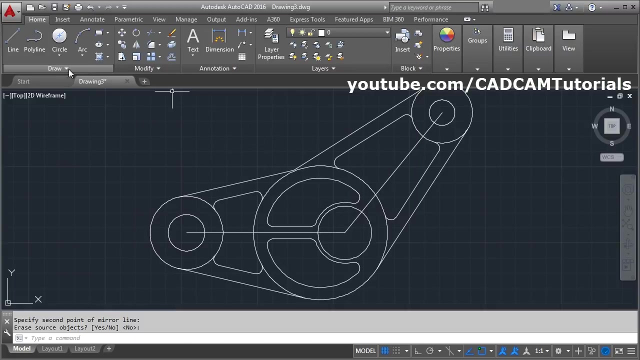 click on mirror. select this portion with the crossing window wherever possible, enter. give the first point of mirror line to the second point. enter then what is remained is this area of circle 7, circle of dia 8 on 30 bcd. create one circle, center diameter. give the center point diameter of 30.. 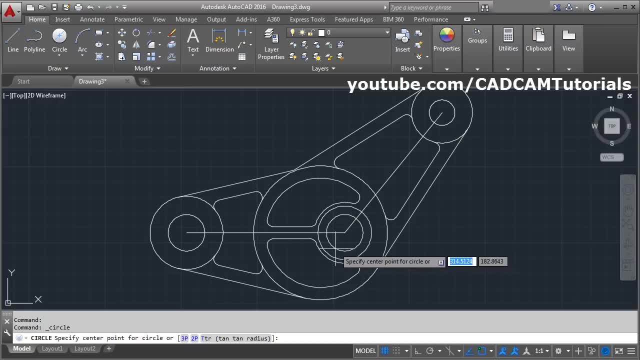 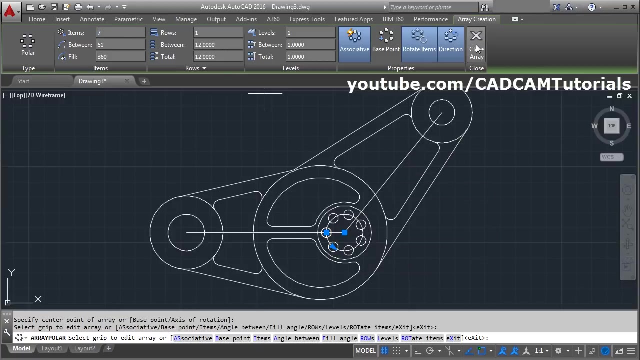 then again center diameter. give the center point, give the diameter of 8, then array it. click here and select polar array. select this circle, enter. then give the center point, then give the number of atoms here to be 7. enter. click on close array, press escape. then erase this reference circle e: enter, remove. 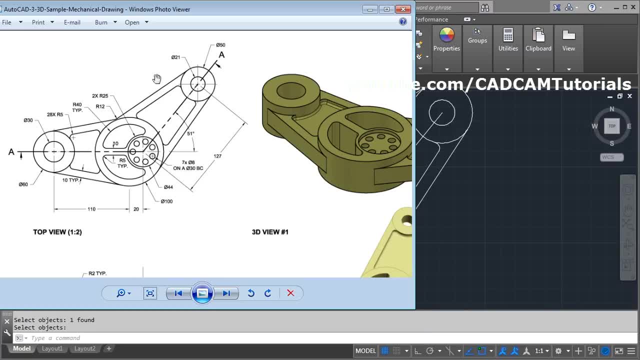 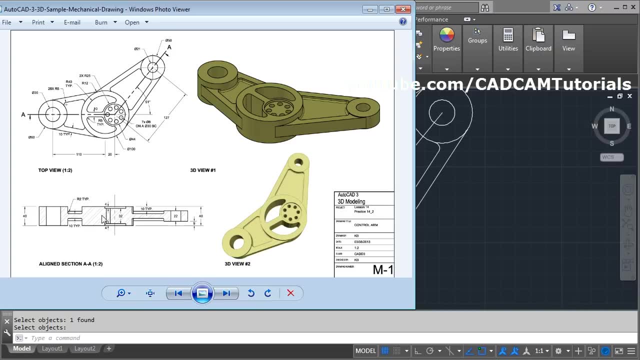 this circle: enter now. this plan is ready. you want to convert this into 3d? now here. actually, this part is symmetric around the center horizontal axis, so we will develop the one side of the object and we will mirror it on the opposite side to complete the 3d object. we will remove this. 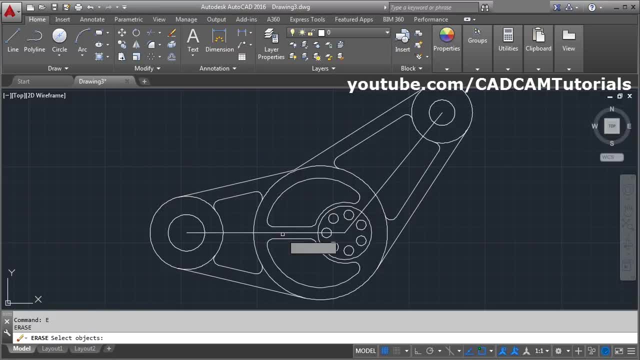 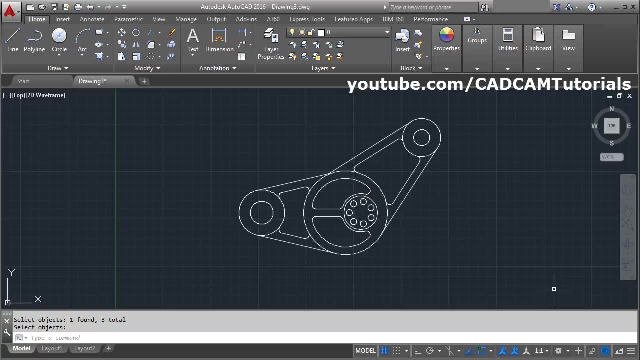 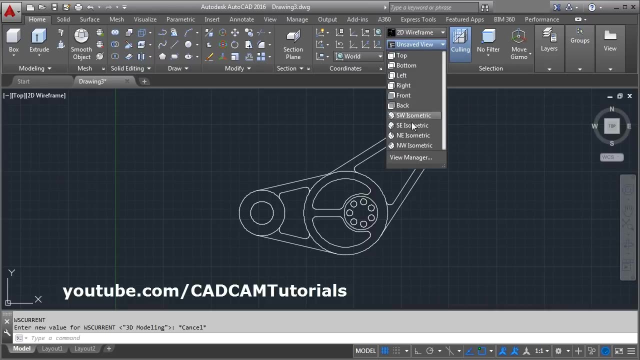 center line. we don't need them. e enter. remove this center lines enter so that it will be easy to convert them into 3d. then to switch to 3d, click here and click on 3d modeling. then click here unsaved view and click on se isometric and click here and select shaded. now this 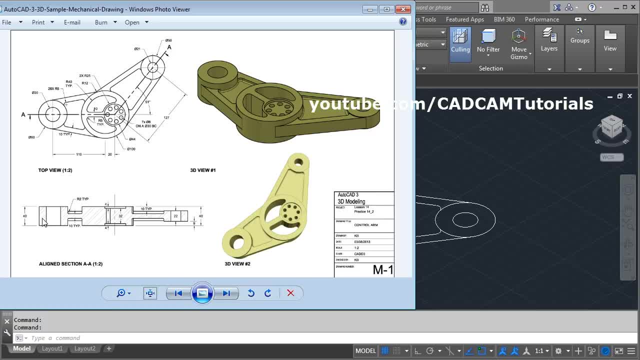 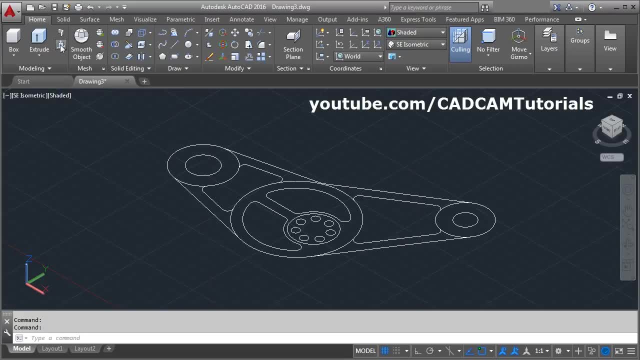 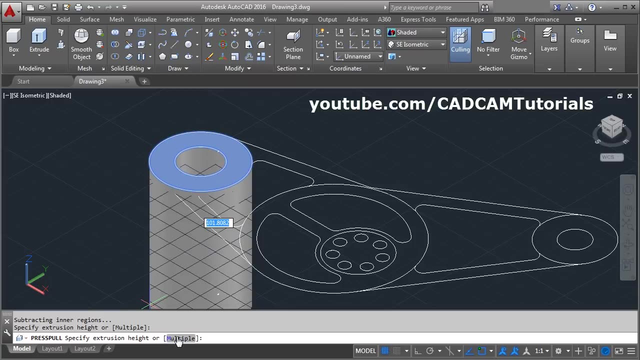 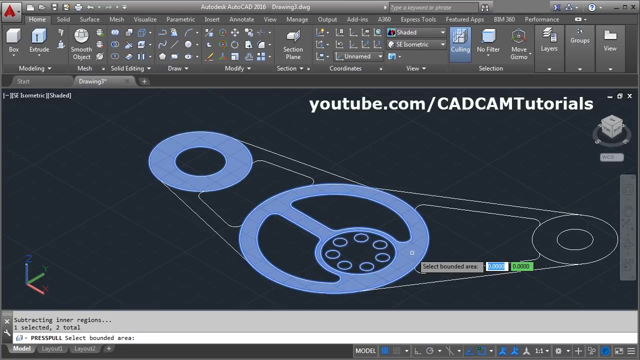 portion is extruded by the distance of 20 from the center and this inner portion is also extruded at 20 from the center. click on press pull. select this portion. then click on this multiple. select this portion, then press enter. take the cursor above and give the. 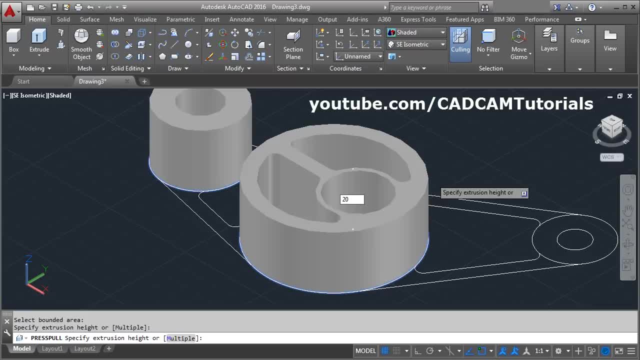 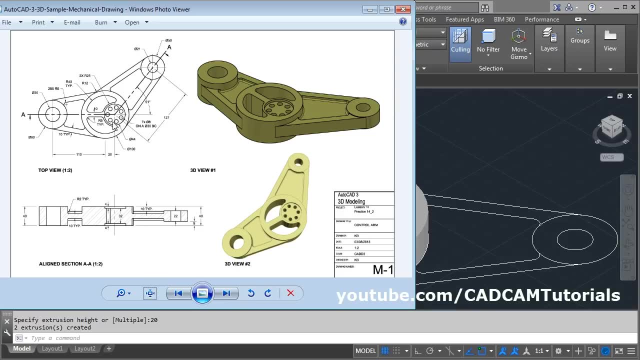 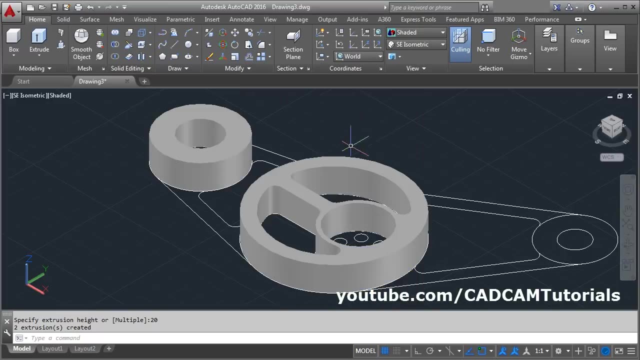 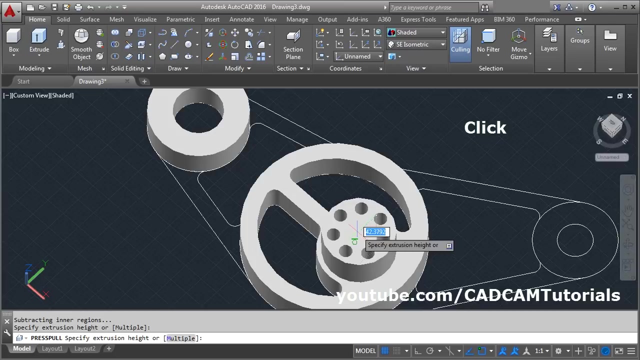 height of half of 40, that is 20. enter. that is this portion, and this portion is ready. then this internal circles: the gap between the circles is 32. that means from the center it will be at a height of 16. orbit it and again, press, pull, take your cursor inside, take your cursor above, give the 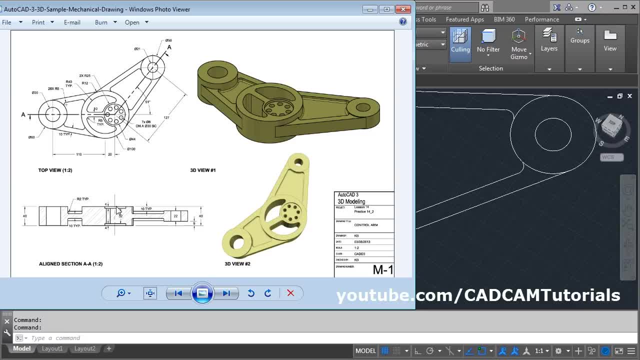 height of 16: enter, escape, then next will be this portion. now to decide the height of this portion. total height is 40. this is 10, and below is also 10. that means what is remained is 20. 40 minus 20 will be 20. so the height of this internal. 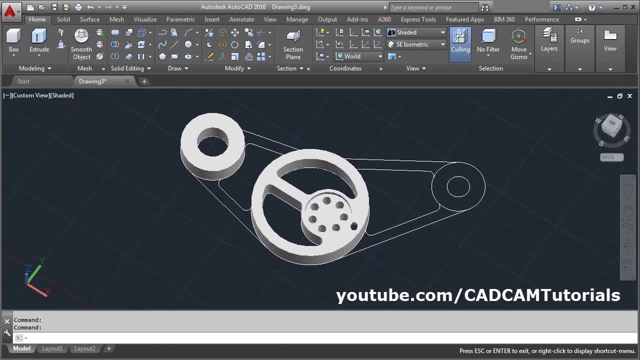 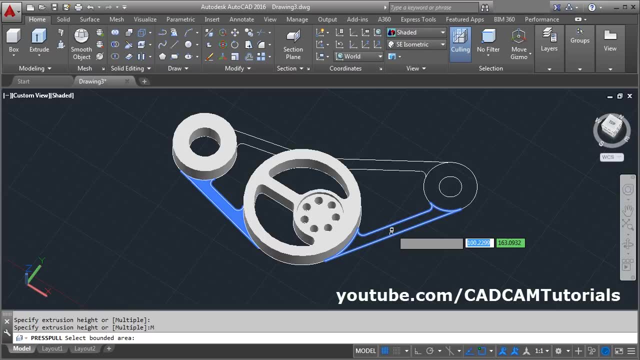 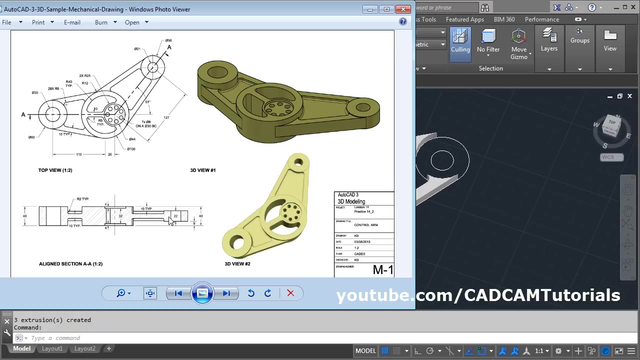 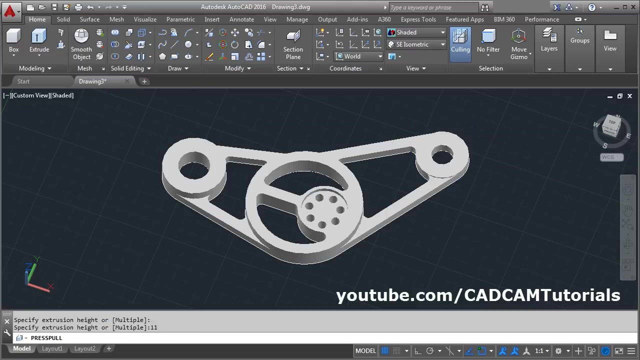 portion is 20. again. take the press pull command, click here. click on multiple. select this portion, this portion enter. give the height of 10. actually, it will be half of 20, that is 10. enter. then this is 22, that is 11. from the center: press pull. select this portion. give the height of 11, enter. 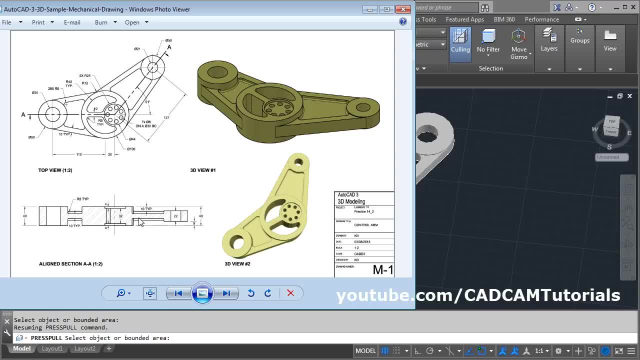 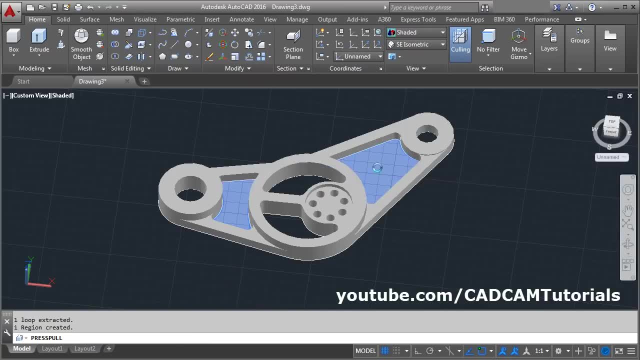 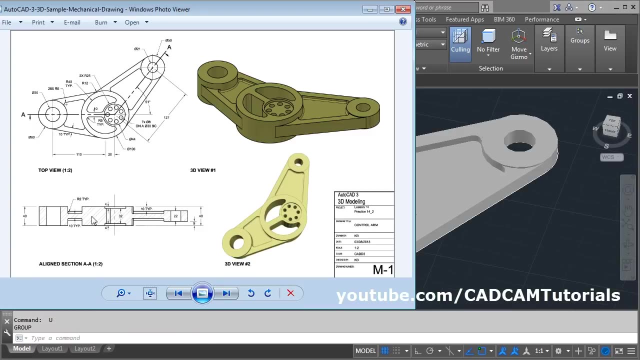 then this inner rib is of 10, that is, 5 from the center. click inside this rib, click on multiple, select this rib, enter, give the direction, give the height of 5, escape. then next is this small fillet of radius 2 on this inside portion here.